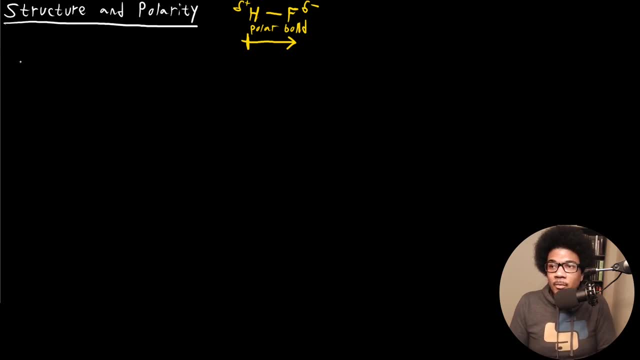 in three dimensions, right? So let's take a really simple example. Let's take the water molecule and look at what we can say about its polarity in the direction of the dipole moment. So for the H2O molecule, right. So again we have H2O, two hydrogens, one oxygen, the oxygen. 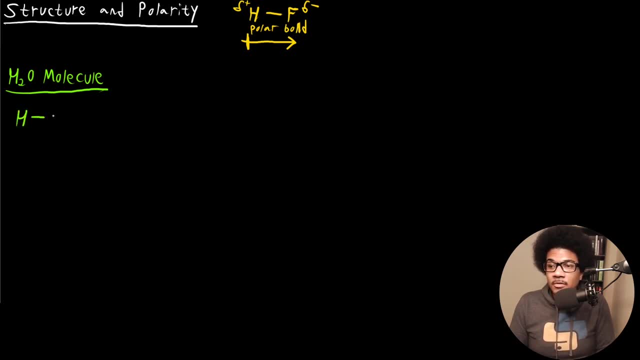 Oxygen is gonna be the center atom. So it has a Lewis structure that looks like this right, Where you got two lone pairs on top of the oxygen. Okay, so if we're calculating a steric number here, our oxygen is gonna be the central atom. 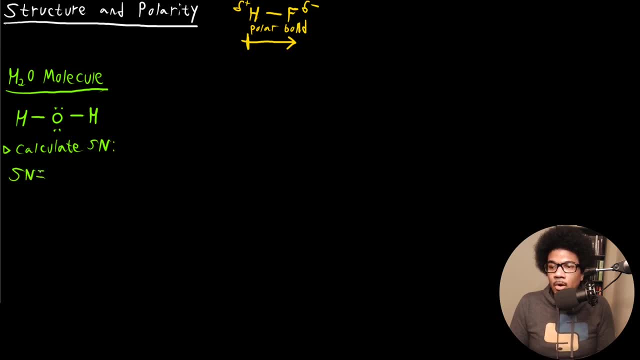 So if we're calculating the steric number, we're going to have two bonds, one to each hydrogen, two bonded atoms plus the two lone pairs here, And that's gonna equal a steric number of four. Now, if you look at your chart, 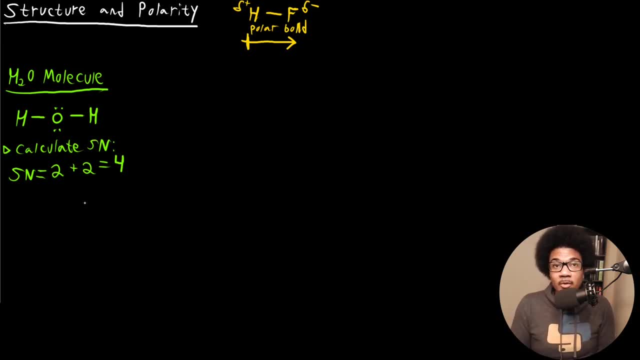 when you have a steric number of four with two lone pairs, that's going to give you a bent structure. So water is going to have the following three-dimensional structure. Let me give myself a little bit of room here. Right, so we got hydrogen there, hydrogen there. 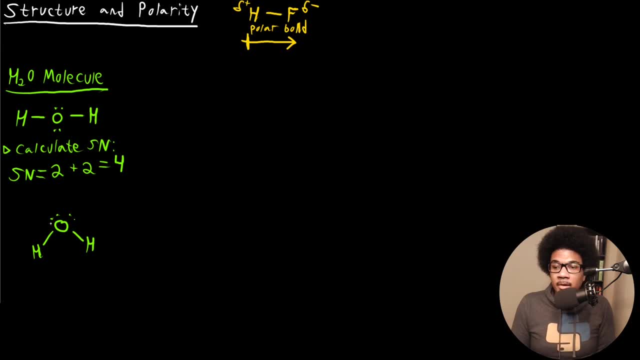 Right. so it's gonna have this bent structure where the electron pairs at the top are taking up a lot of space and they're bending those bonds to the hydrogen downward. So this is going to be the three-dimensional structure for water. Now what about its polarity? 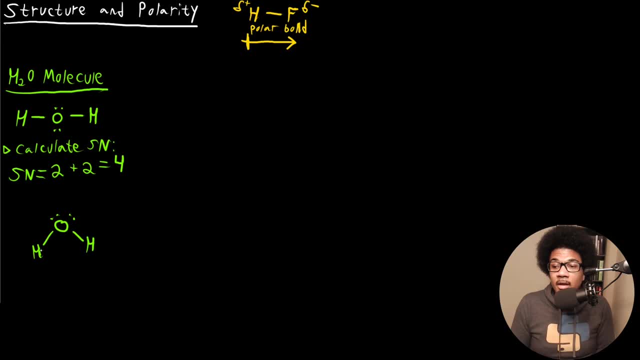 We know that both of these bonds are going to be polar bonds, right? So you're going to have a partial positive at each individual hydrogen and a partial negative at the oxygen atom, right? So when we talk about the directionality of the dipole, 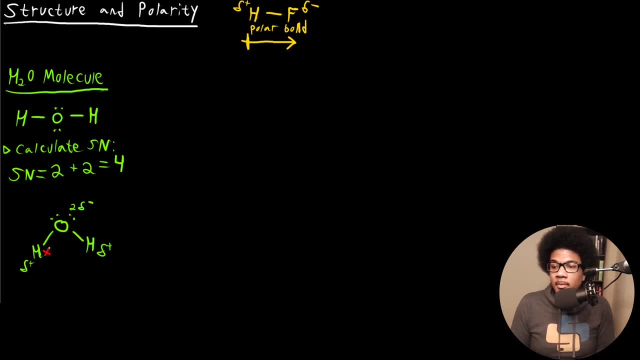 right, we know we're gonna have, you know, a bond dipole that points this way here and a bond dipole that points this way here, right, And so what we can start to talk about is the overall direction of the dipole moment. 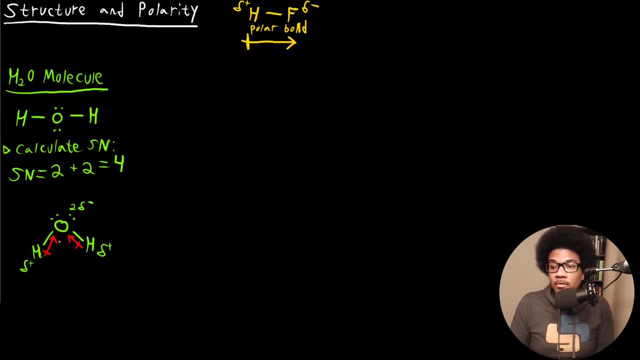 for the molecule right. Since these are both pointing upwards toward the oxygen, we can have a total molecular dipole moment that's pointing this way right. So you can think of this how you might think about vectors in algebra, right, The two vectors are kind of you know. 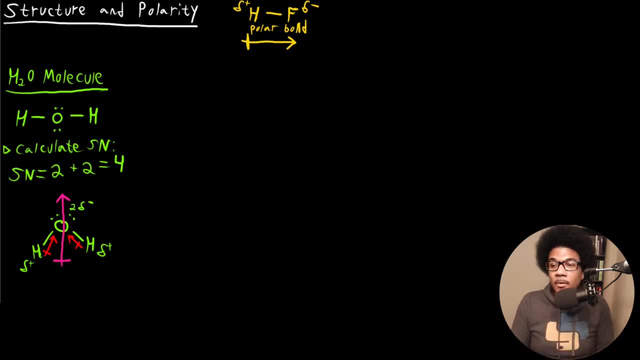 in a direction where they're adding together and so they're going to form a molecular dipole that points in this direction with respect to the framework of the water molecule, because of the direction of these two bonds. So we can start talking about the directionality. 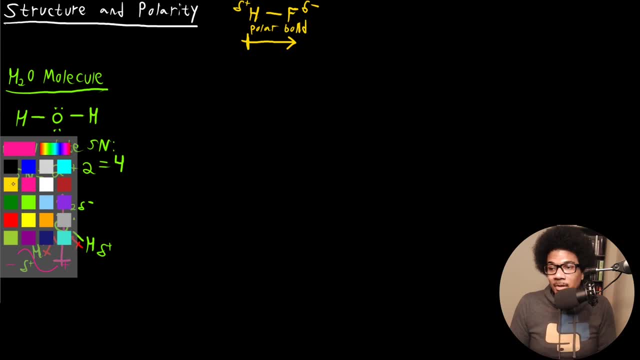 of this polarity. right Now let's look at another example here, and the example I want to look at is Xenon XEF4, right, Classic example. really cool story behind this: Noble gases thought to not react with anything. 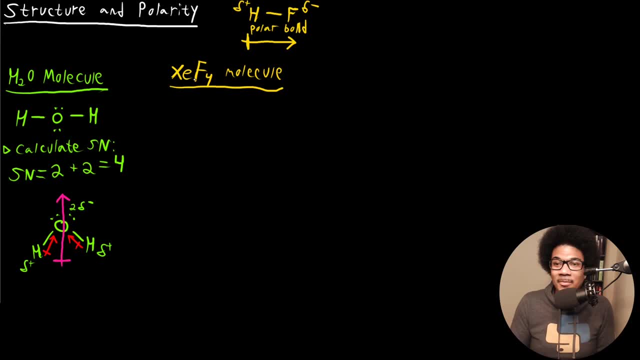 and somebody won a Nobel prize by reacting Xenon with a bunch of halogens, and the rest is history. But that's, that's the XEF4,. right, That's the XEF4 molecule. So for XEF4, it has the following Lewis structure: 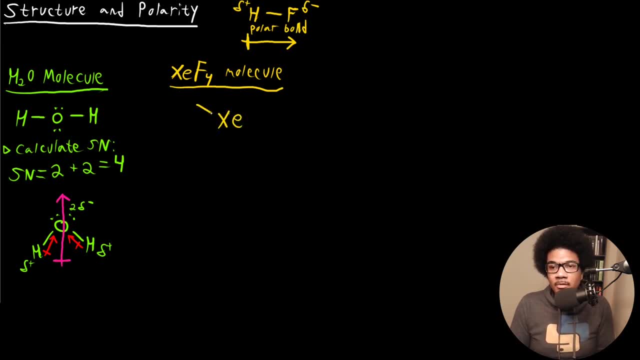 I won't go through all of the details here, just because I really want to focus on the polarity conversation, but it has the following Lewis structure: So of course we got lone pairs around our fluorines and we still have two long pairs around our fluorines. 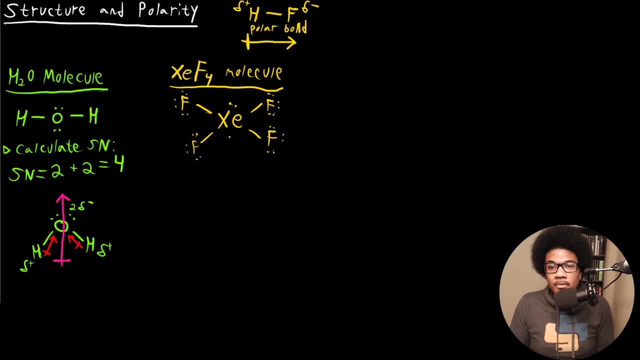 and we still have two long pairs that are outstanding here, And so we put those on Xenon. Xenon is well below period three and so it has those close by D orbitals in order to accommodate more electron pairs, So it's happy with this expanded octet. 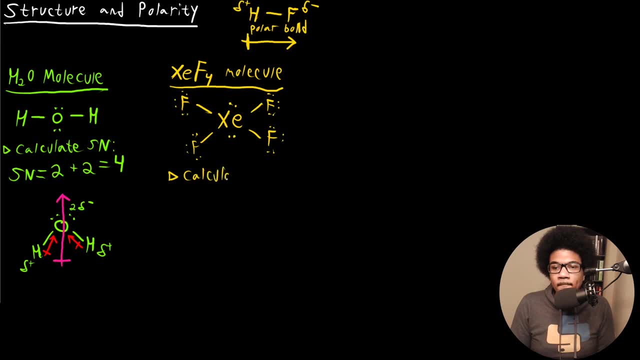 So that's our Lewis structure. So now we want to calculate a steric number. All right, so we calculated a steric number. Steric number: So we have four bonded atoms here, with each fluorine bonded to the Xenon, and that's going to be two lone pairs. 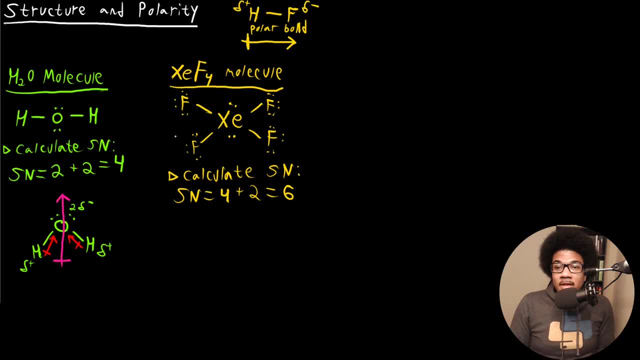 So it's going to give us six. So if you look at the table, when you calculate a steric number of six and you have two lone pairs on the central atom, that's going to give you a square pyramidal structure, right. 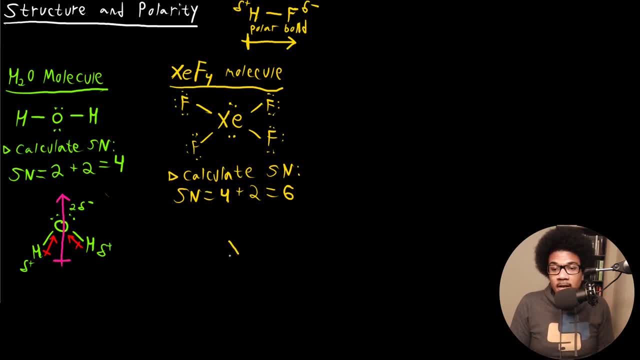 So basically, it's going to be a square with Xenon at the center of the square, right. So I'm just going to draw these here without the lone pairs present. Okay, so if we investigate these, just on the individual bonds, right? 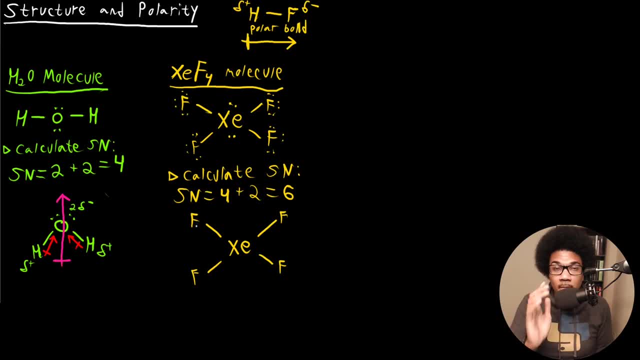 We're going to have polar bonds all around. Fluorine is much more electronegative than Xenon, So we're going to have a partial negative at each of these fluorines, Right And so for each of these- and I'll put a partial for partial- positive here at Xenon- 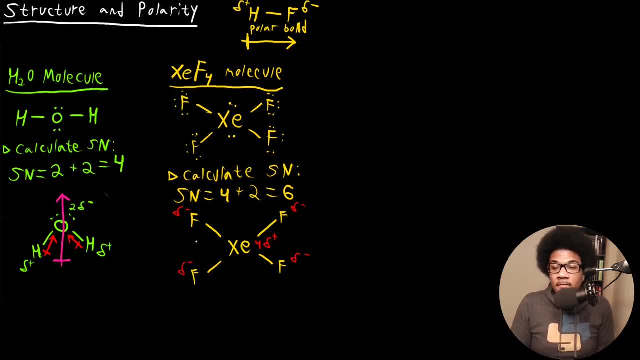 right. So all of these are going to be polar bonds. They're going to favor the fluorine right. So we're going to have polar bond dipole here, polar bond dipole here, polar bond dipole there, polar bond dipole there. 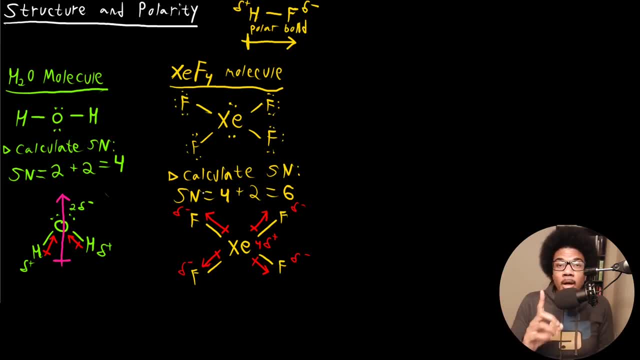 Right. So we got polar bonds all the way around, but I want you to ask yourself: do we have a total molecular dipole And, if so, what direction is it pointing in? So what I wanted to drive home with this example is that you can have molecules where you have polar bonds. 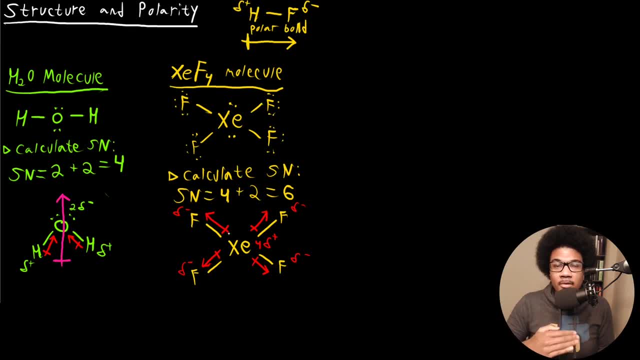 but there is no overall polarity for the molecule, There's no overall net dipole. And this is the perfect case, because you have all these bond dipoles are going to cancel each other out, right? You see that this is going in the exact opposite direction. 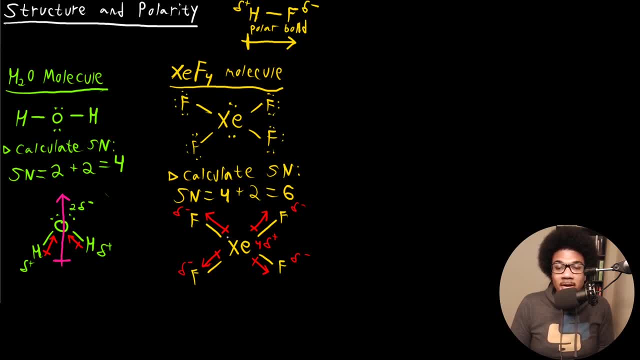 of this one, This fluorine bond, is going. the dipole is going in the exact opposite direction of this one, right? So we actually won't have an overall molecular dipole here for Xenon tetrafluoride, because all of these dipoles are going to cancel out. 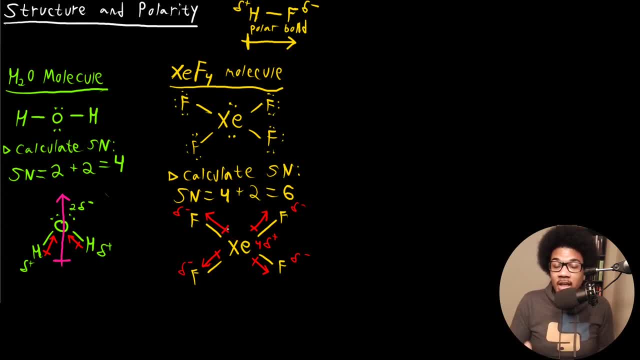 And that is a direct consequence of the shape of this molecule, Since it's square, pyramidal, these dipoles are pointing into the dipole, They're pointing in the exact opposite direction of one another, And so we don't have a net molecular dipole, right?